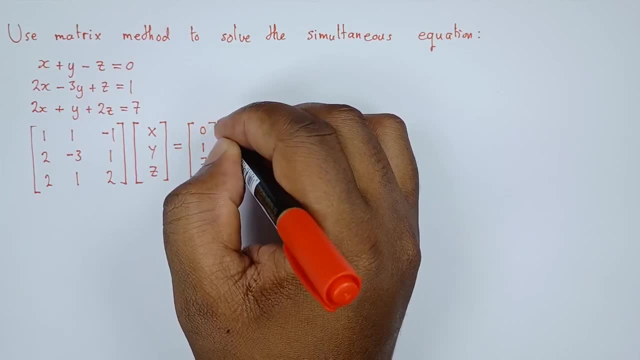 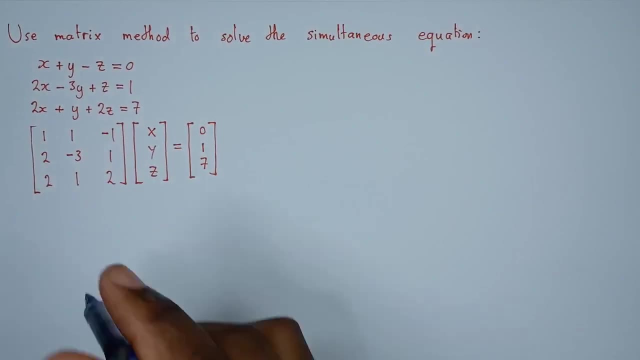 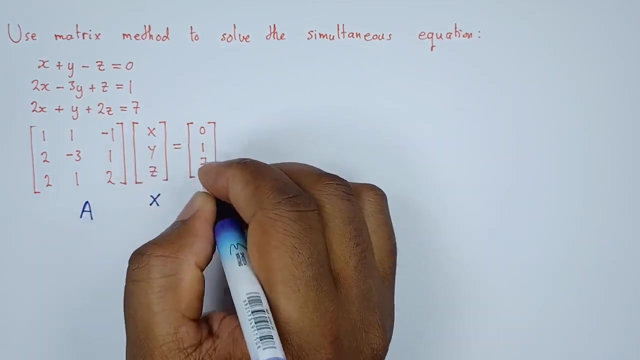 are 0,, 1, and 7.. Okay, So, now that we have this, we're going to call this matrix A. This matrix, we'll call it, let's keep it. X. This matrix, we'll call it B. 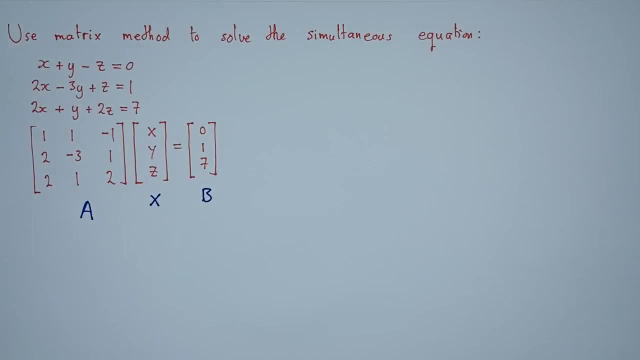 So we're looking for the values of X, Y and Z, meaning that we're looking for the matrix X, So AX is equal to B. But since we're looking for the matrix X, we're going to say X is equal to A inverse times B. 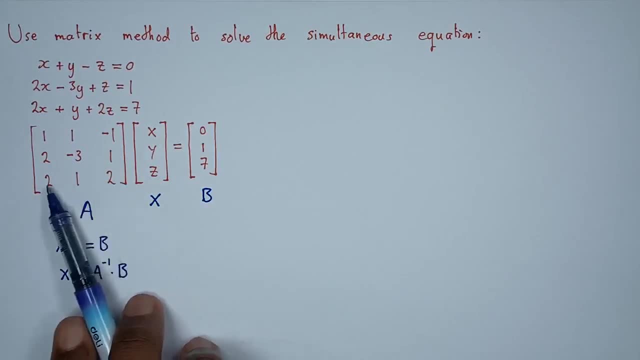 So in other words, we have to find the inverse matrix of A, multiply it with B, then we have the matrix X. So finding the inverse matrix is a bit of a lengthy process, but let's go. So at least you understand now how to solve this. 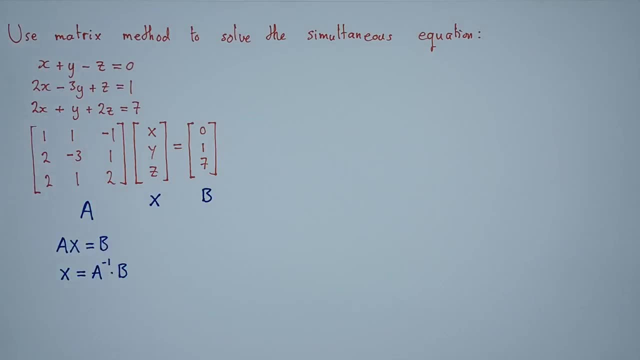 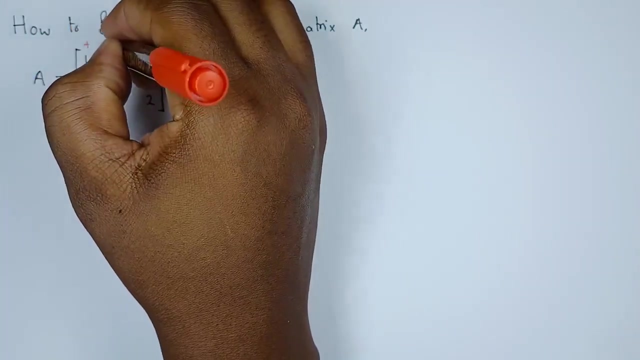 So let's start by finding matrix A, then we can come back and find matrix X, So let's find the inverse of matrix A. The first thing we're going to do is we're going to set up a plus, minus, plus. 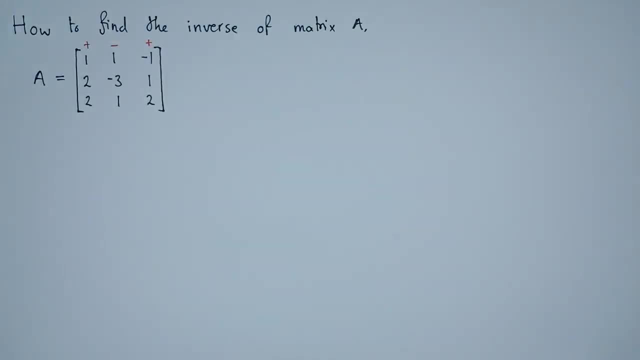 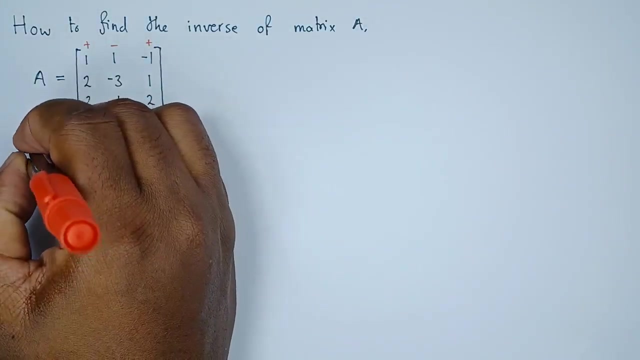 So, in the process of doing this, we're actually trying to find the determinant of this matrix A. That's the first thing to do. So, to find the determinant. what we're going to do is we're going to say that A- meaning the determinant of A, is equals to 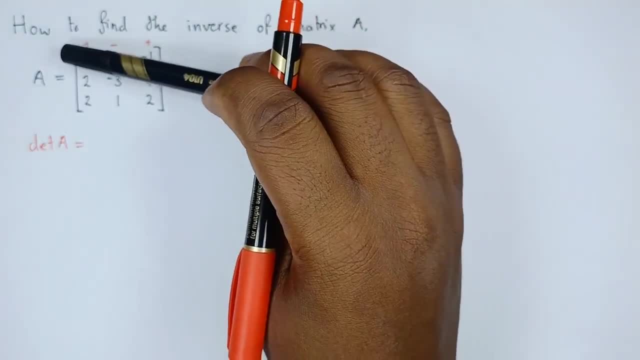 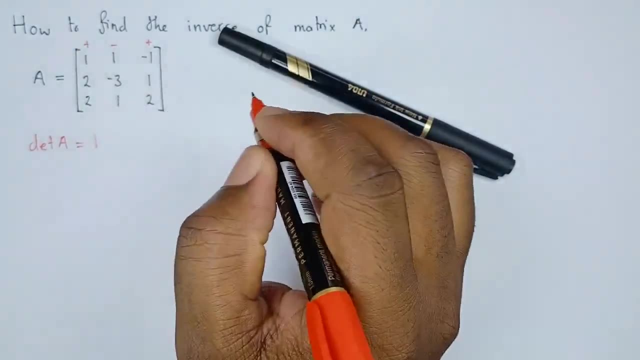 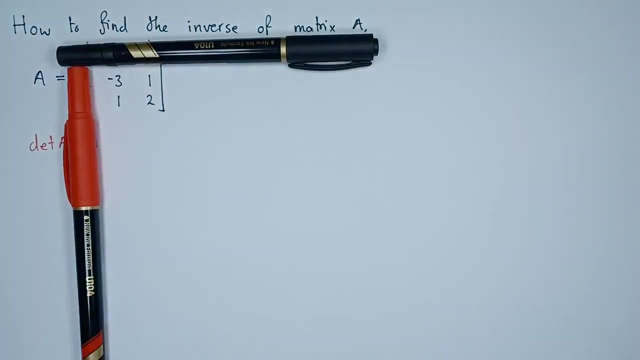 So getting the values in the first row, which is one, one negative one, we're going to set them up like this: We start with the one, then we form a two by two matrix that is formed when we cover the row and column. 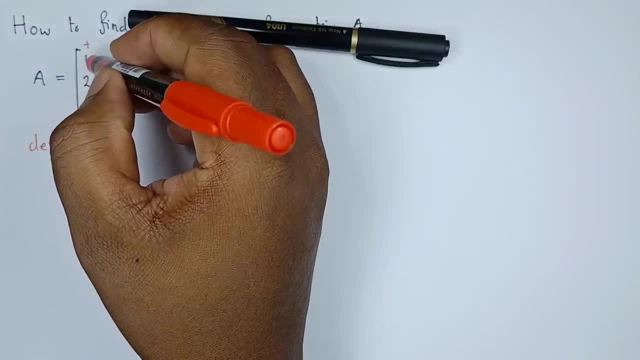 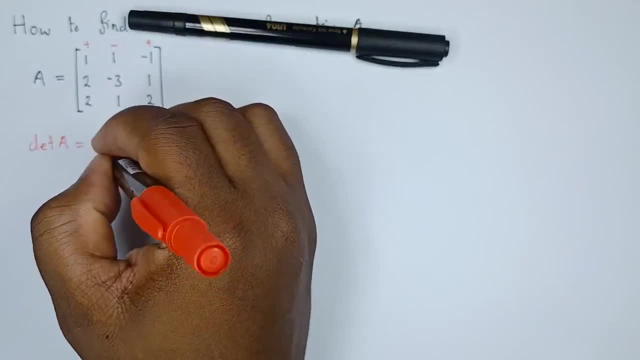 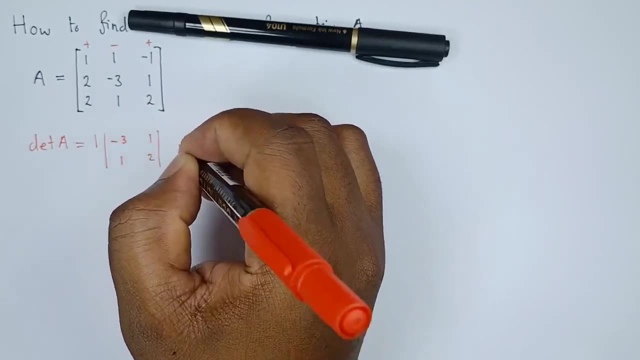 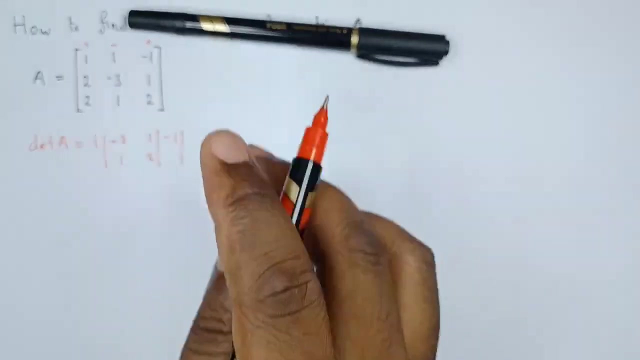 So if we get one, we hide the two by two matrix and we get one. Hence we remain with negative three. one, one, two. Then here we have a minus, so we say minus one, the two by two formed. 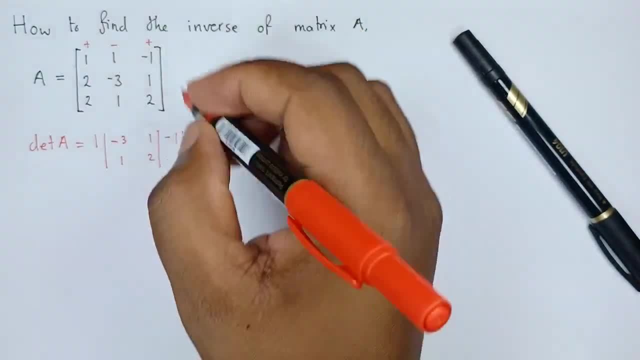 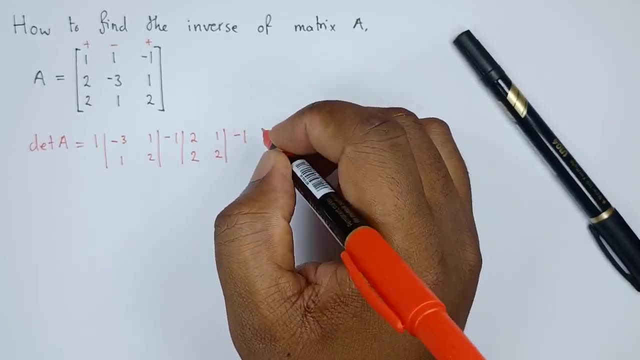 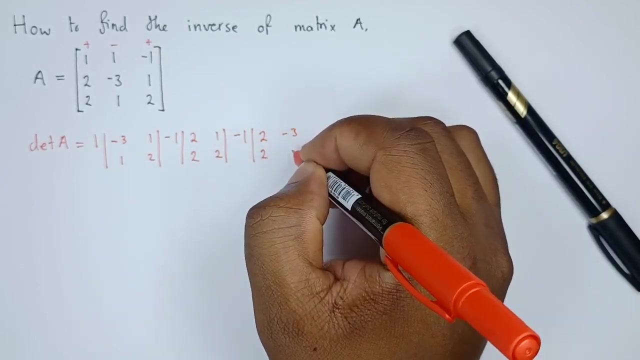 If we hide the row and column for this one, we're going to get the matrix two, two, one and two, like that. then, lastly, we have negative one, this negative one that we have here. so the two by two formed will be two, two negative three and one. so so that you understand it, how we're coming up with this, 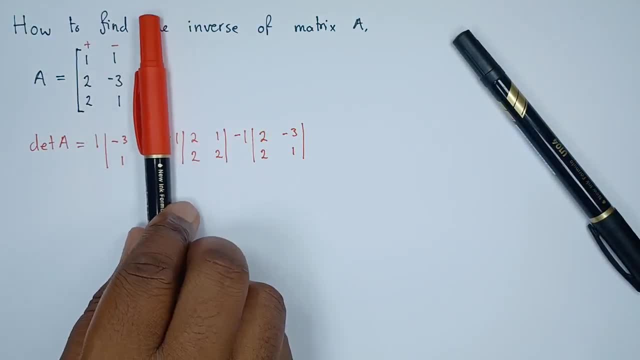 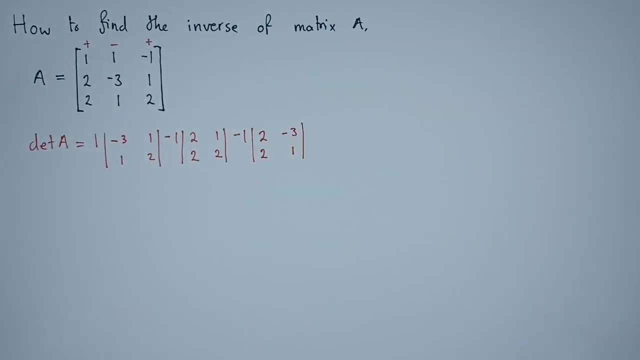 matrix is we are hiding the row, the column which is this one and the row which is that one. hence we just eliminate the four values which of course form the two by two. so it's just a matter of finding the, the determinant of the two by two. then we can proceed and find the determinant for. 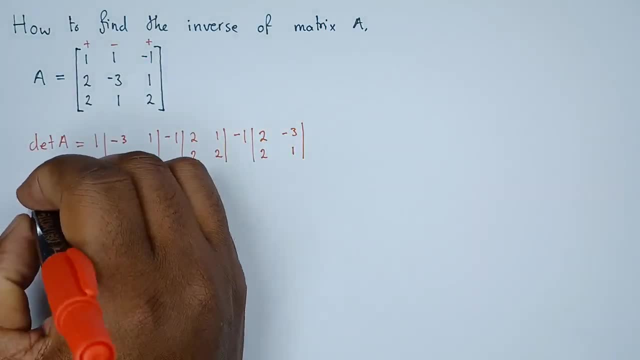 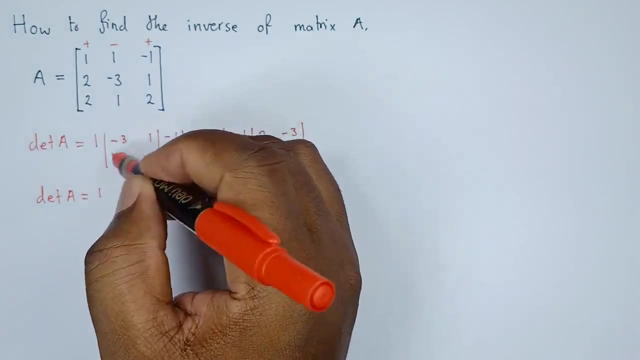 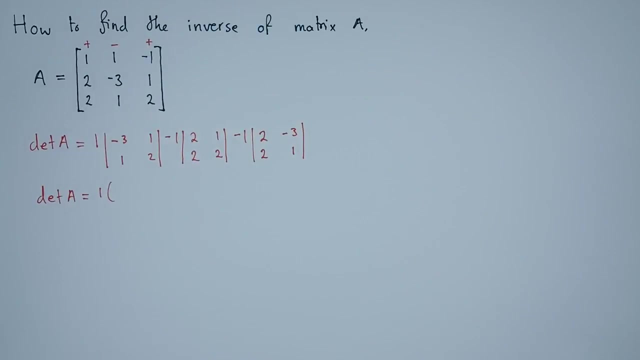 this particular three by three, of course. this is the whole process. so determinant of a will be equals to. we have one here. let's find the determinant of this two by two to do that we shall say major diagonal minus the minor diagonal, so negative three times two we get. 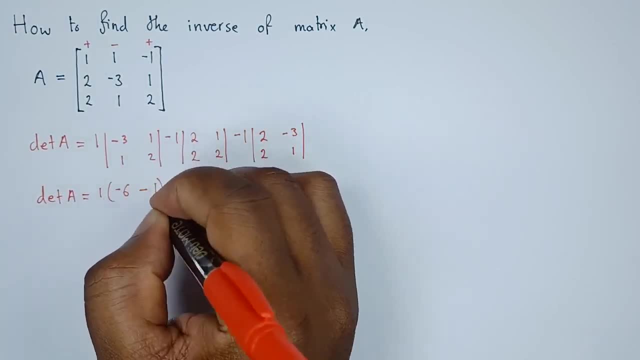 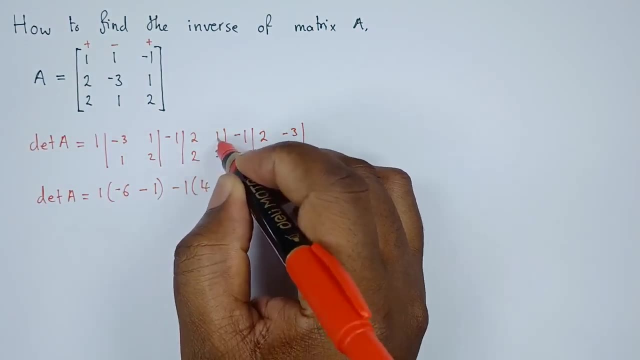 negative: six minus one times three minus a whole. so we will get a two by two and we have a two by two, and then we willnerside: one is just one minus one. this one here two times two is a four minus two times one is a two. 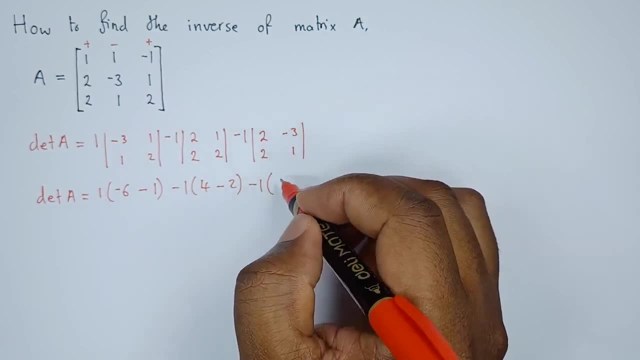 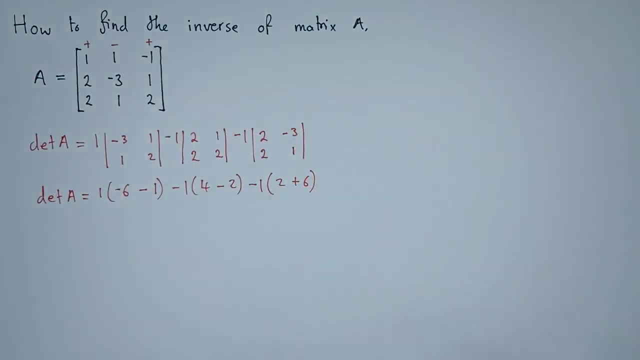 minus one. two times one is two. two times negative. three is a positive six. remember this negative. then replace the negative, since we're subtracting them here. so get a positive value. then from there we're going to say: the determinant of a or that a is equals to 1 in the brackets negative: 7. 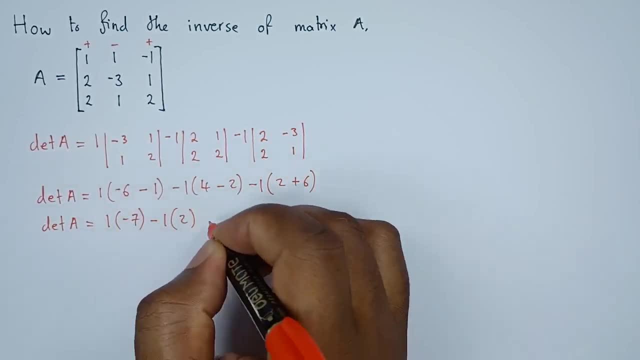 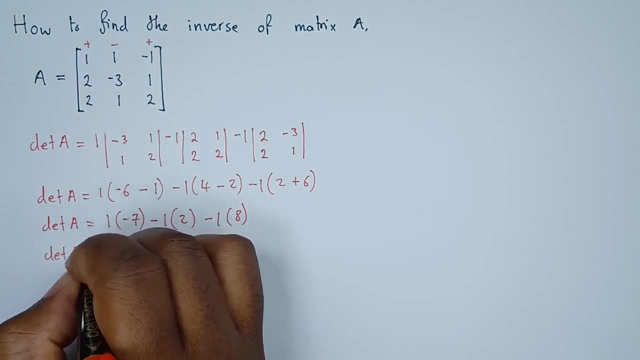 minus 1 the brackets, we have a. 2 minus 1 in the brackets, we have 8. so what we get, so that a will be equals to negative 7 minus 2 minus 8. so if we put everything together, we'll see that that a simply. 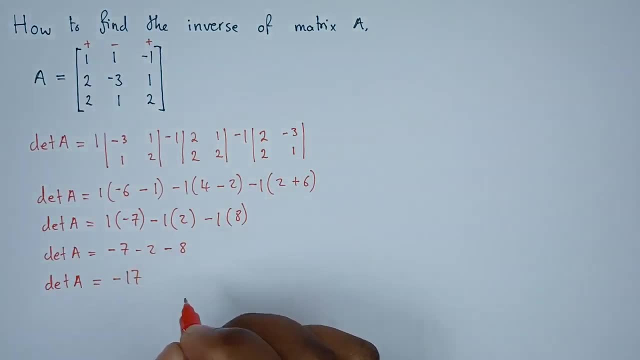 equals to negative 17. okay, so now that we have the determinant, what we need to find is the adjoint. to find the adjoint. we're going to find the, the cofactors, and we can see how we can find that joint. so let's go ahead and do it. 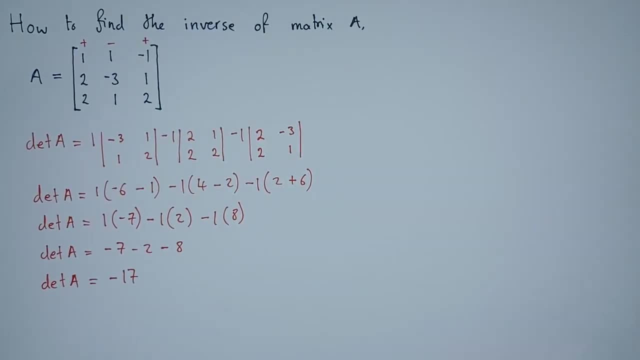 okay, so let's obtain the cofactors. so let's do this. let's first start by demarcating. so we're going to create a very big matrix, and that big matrix will be formed like this. the first thing we're going to do is let's just write. 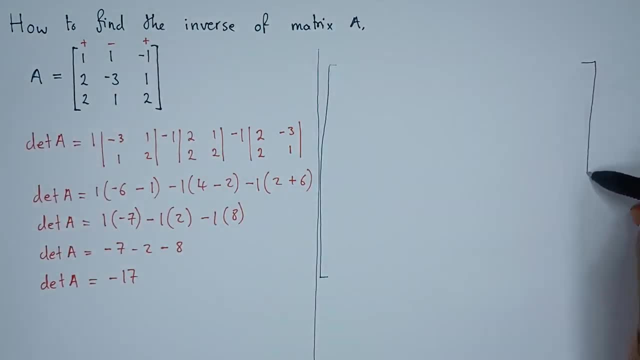 the matrix. okay, something like this: I hope everything is visible, okay, so, just like we're doing for the determinant, we're going to do the same, such that we have nine positions, nine values. well, that is rows, and the rows are the columns. everything is giving us up to nine in terms of the values. 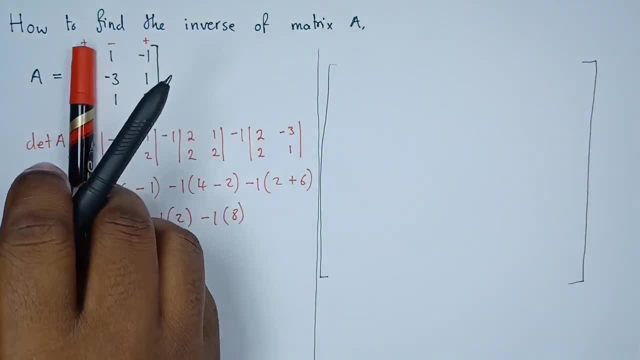 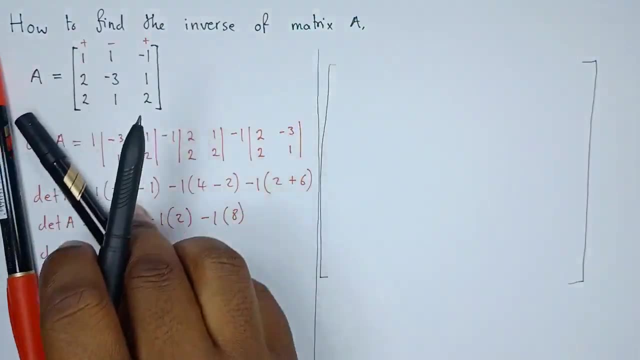 okay, so we're going to create a very big matrix, and that big matrix will be so at each position we are going to create a two by two matrix. so, starting with the position, the first one, which is one, we know that that position is one that will form a two by two. here. we'll have another two by two here, another two. 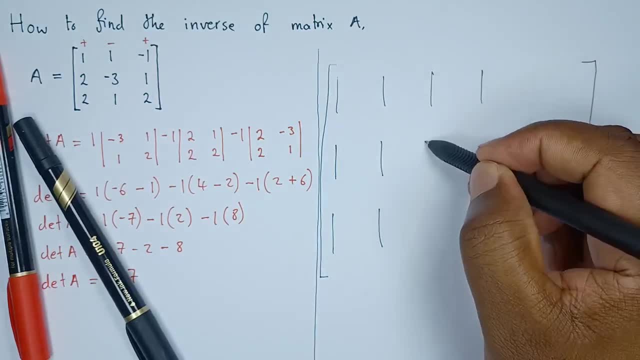 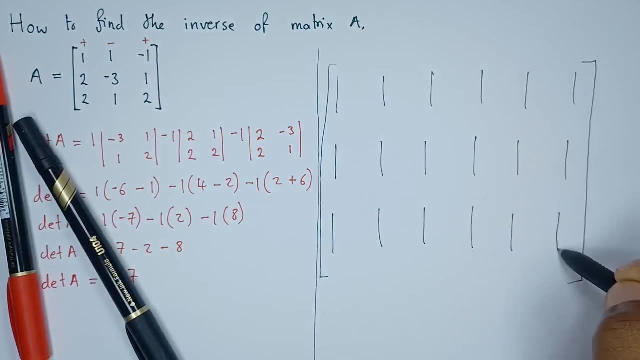 by two here, another two by two here, another one here, another one here. so we need nine of them. so these are just the determinants, of course, or the two by two, the two by twos, and then we're going to find the dissimilants. so, at each position, 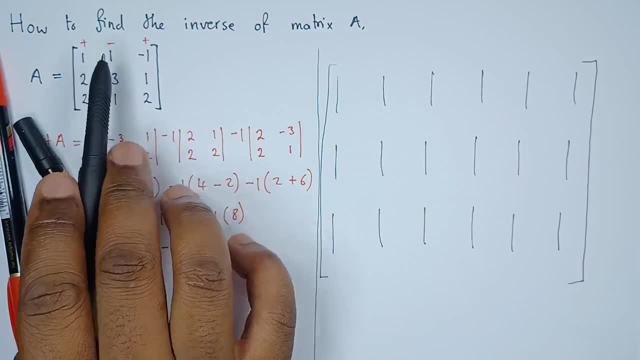 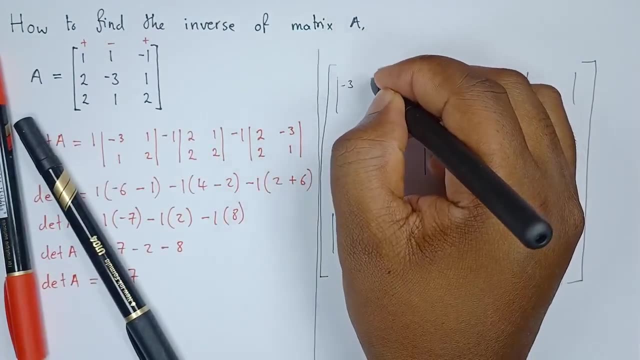 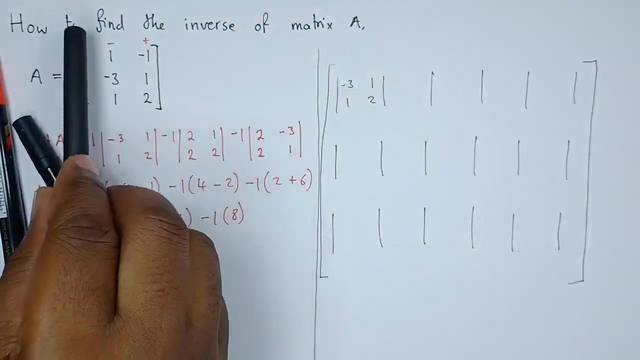 starting with position one, how do you form the two by two? we're going to hide the row and column for this one, hence the values that remain. we have negative three: one, one and two. if we get this position for two, then we hide the row and column for that particular two. so what remains? we remain with one negative. 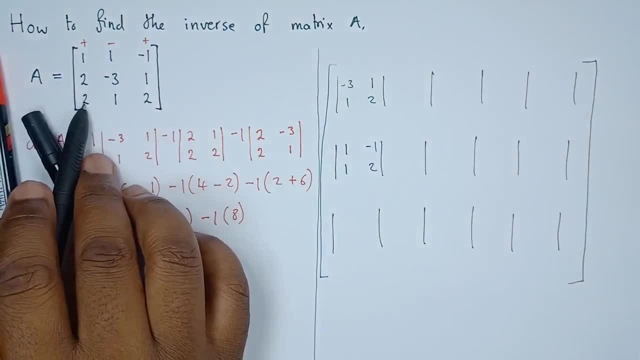 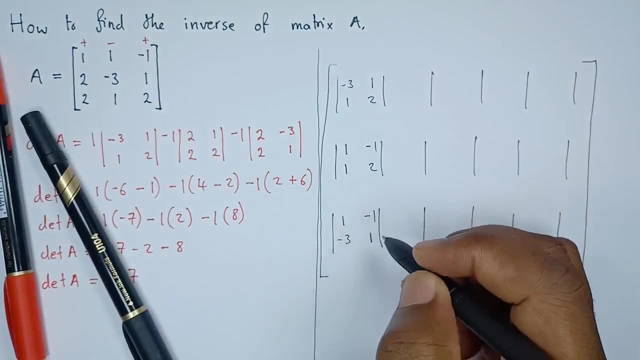 one, one and two. we come to this two here. same thing, hide this two, two, and there's oh that one is still one, one, two, two. like this: we see that if we close this box, the row, and column what remains, one negative one, negative three, one. so we're done with the first. 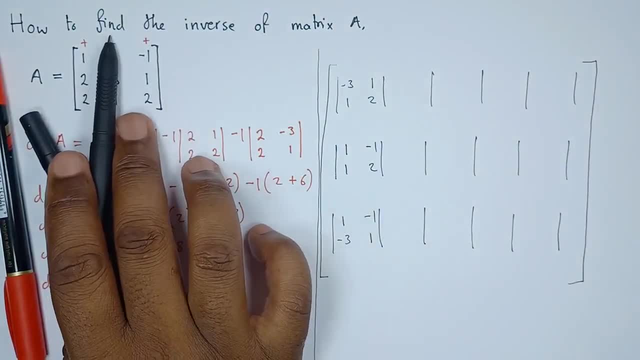 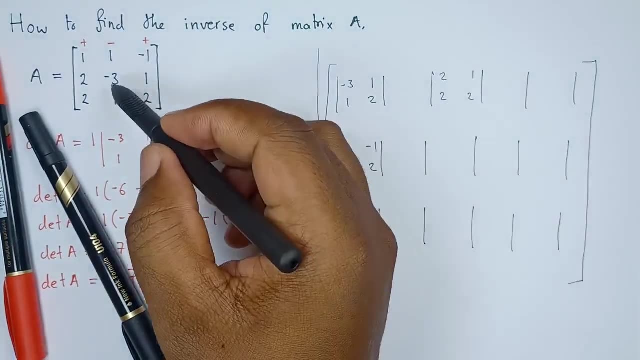 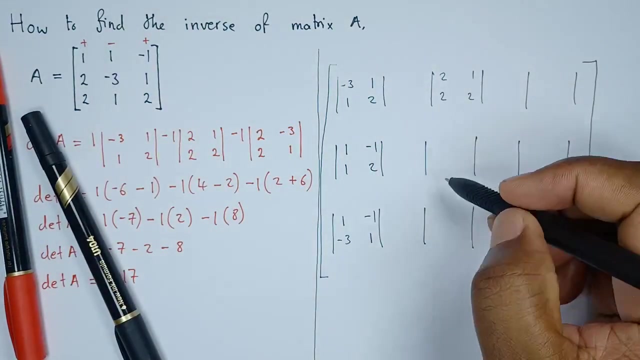 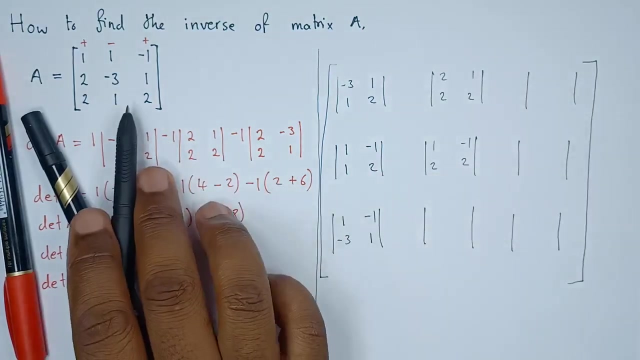 column. let's go to the next column. so for this one we hide the column and row what remains: two, two, one, two. we go to the central three. so we hide the column, the row and column for that three. so what are the values that remain? we have 1, 2 negative, 1, 2. we move on to this one. here we hide. 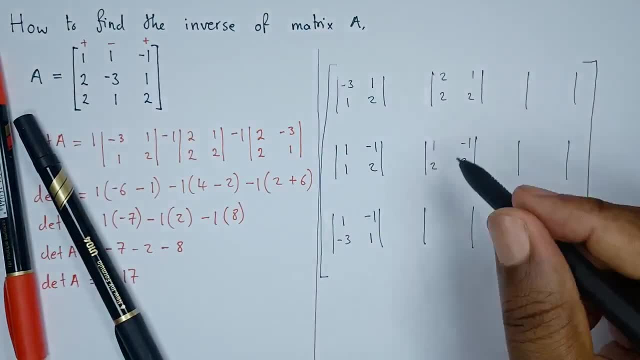 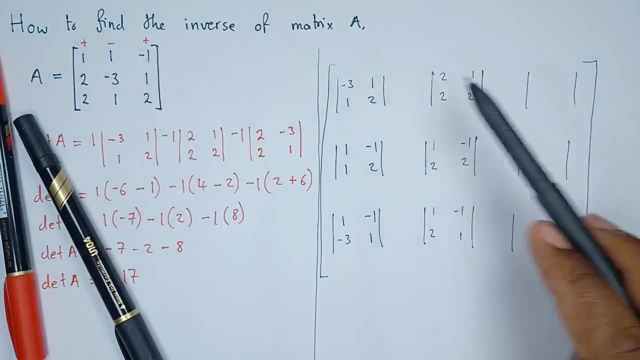 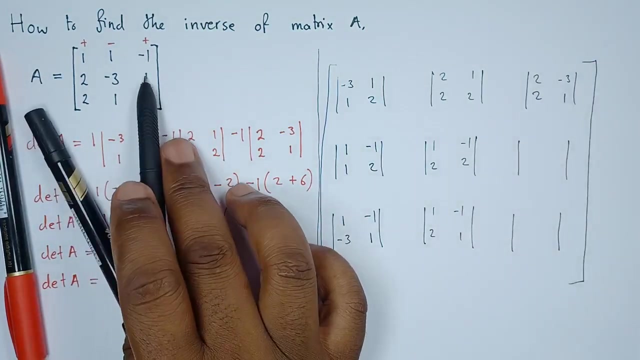 the row and column what remains, one, two negative one, one. I'm sure you get the idea now. so if we go to this one which is at this position, the 2 by 2 form will be 2, 2 negative 3, 1 at this one here. 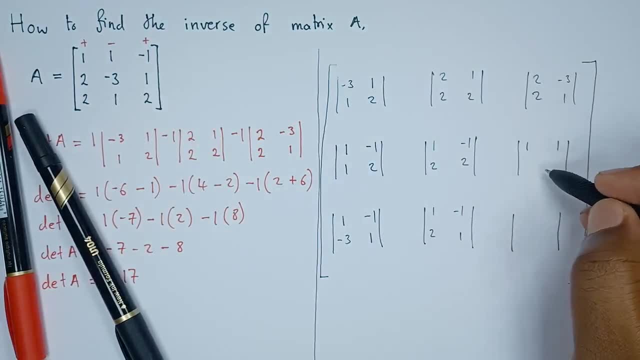 the 2 by 2 form will be: 1: 1, 2, 1, the last one, which is this: 2. the 2 by 2 form will be 1: 1, 2, negative 3. okay, so now it's very vital that you don't forget this: if you form whatever formed here, don't forget the signs you. 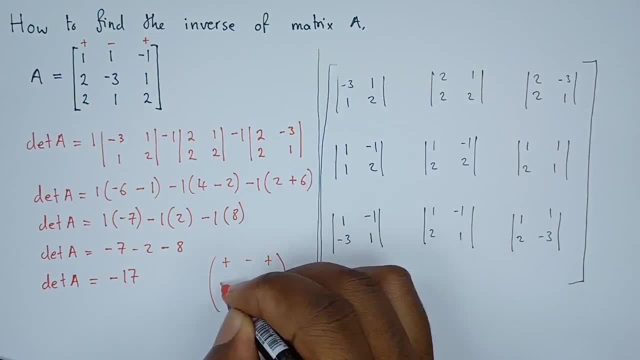 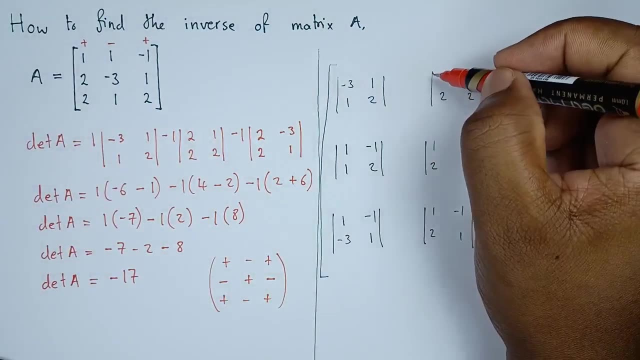 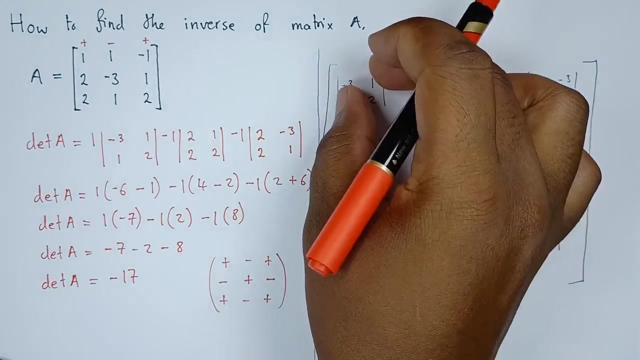 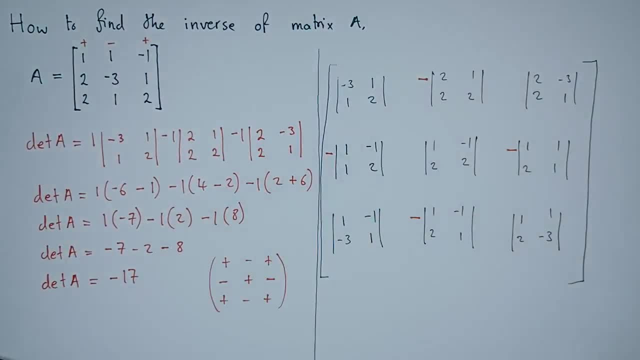 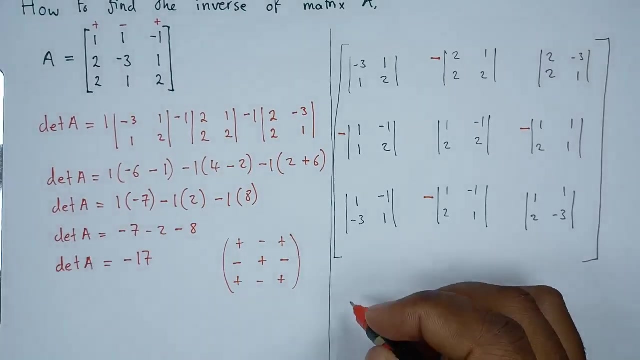 it with a negative according to the signs that have been presented here. so let's find the the 2 by 2 determinants at each position. this is what will help us find the adjoint of this particular matrix so determinant at each position. so let's start at this position. we'll say major. 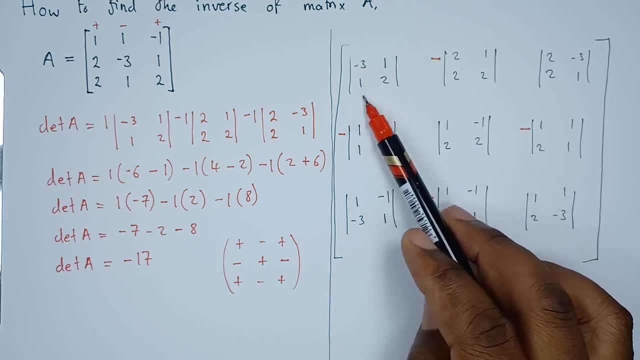 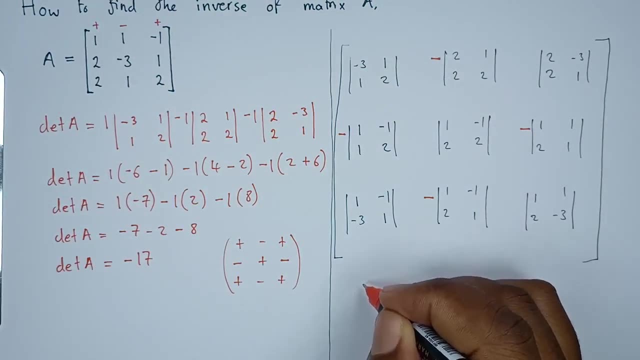 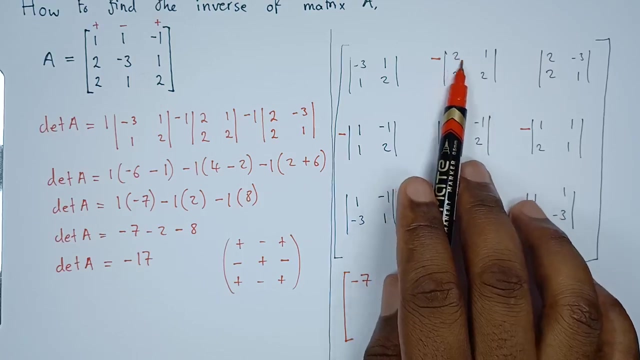 diagonal minus minus. so that is negative 6 minus 1. remember negative 6 minus 1, which will just give us should be a negative 7. okay, from there we come here, so it'll be 4 minus 2 or minus 2, which is a 2, but we have a negative outside. 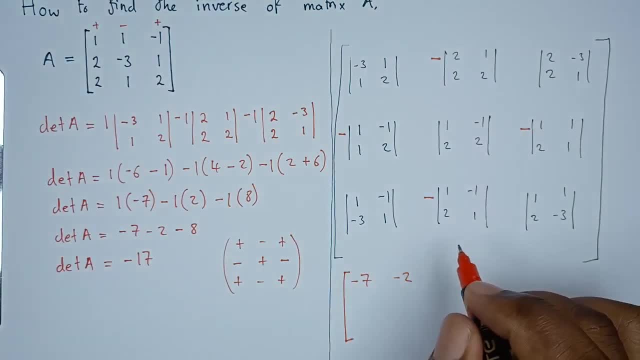 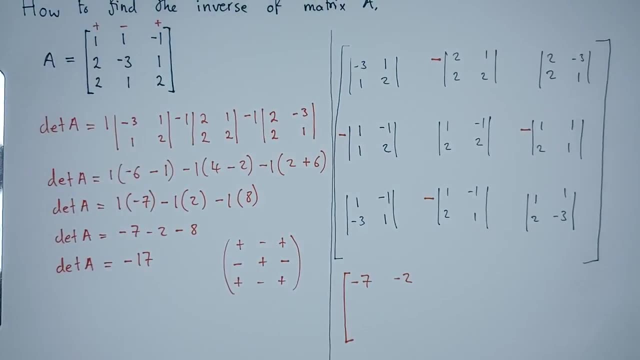 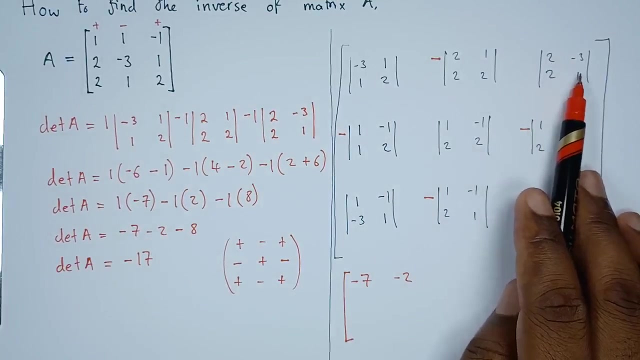 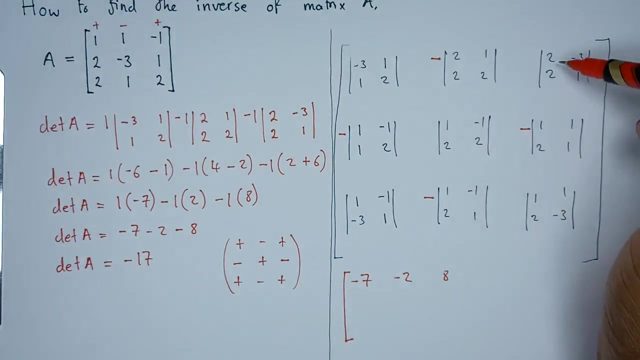 so negative 2. move on here. we say 2 minus, sorry, 2 times 1, that is 2, so 2 minus negative 6, or rather two plus six. so just get eight, now that eight i believe must be. is it negative or positive? let's go through. should be positive, yes, positive. 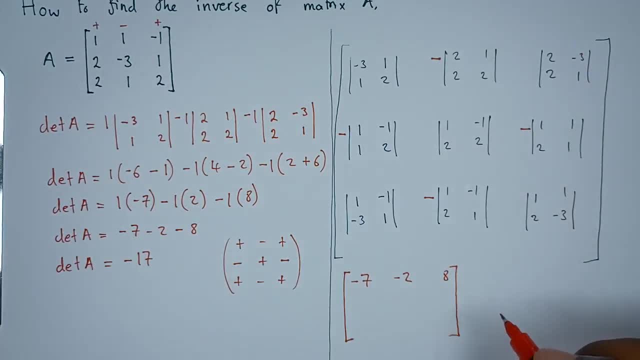 okay, so we have that next thing here. this will be two plus one, two plus one, hence we get a three, but there's a negative outside, so we'll get negative three. when we come here, it'll be one minus three, hence we get negative two. like that we come here or let's do the central. 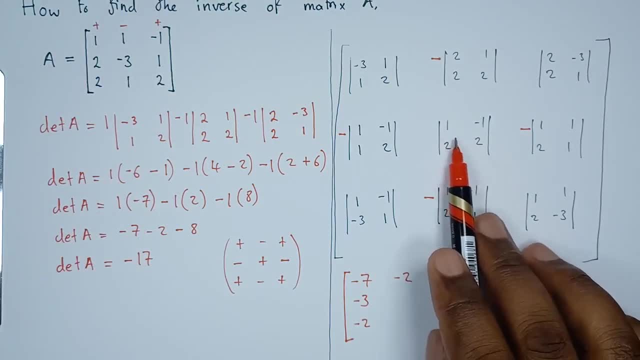 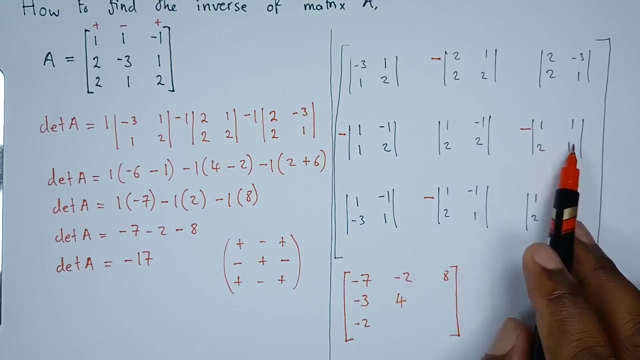 we'll have two minus negative two, so two minus negative two. hence we just get um four. we come here. we'll have one minus two, so one minus two is um negative one. then, with this negative, then we'll have a positive one. we come here. this will be one minus negative two, one minus negative two. hence we'll obtain: 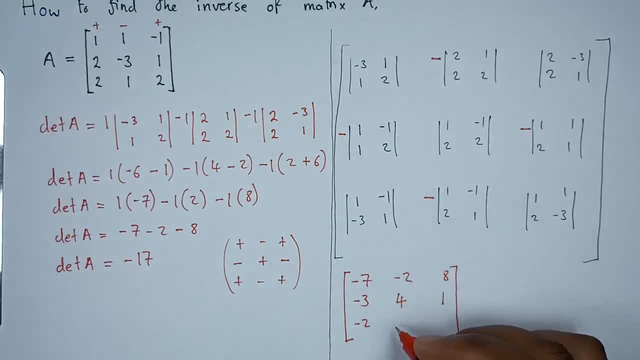 a three inside, but with that negative. hence we have a negative three. like that, we come here. well, we go ahead. we go to the column we Darjeel and we radian divide means negative one five. so so so here we have the column, the column والق. so this will give us a negative three minus two. so negative three minus two, we get a negative five. Okay, so now what we're going to need to do is, we suppose, to transpose this. so let's take the transpose. so if we transpose this we're still tone. so of course, transposing simply mean the ROE becomes the strategic column again. we're going to need two columns: we take the column and we give the column two. 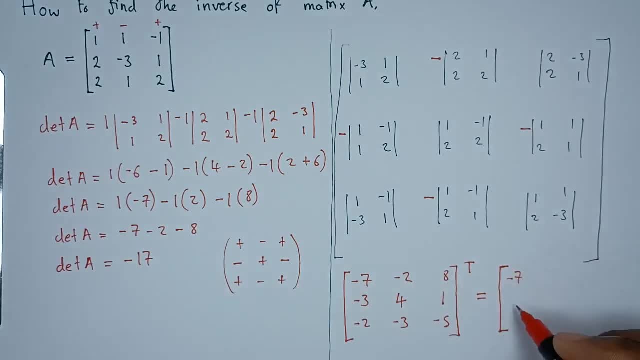 the first row is negative 7, negative 2, 8. this row becomes a column. the second row is negative: 3, 4, 1. third row: negative 2, negative 3, negative 5, like that. okay, there we have it. so what we've obtained? this is the adjoint of this material. 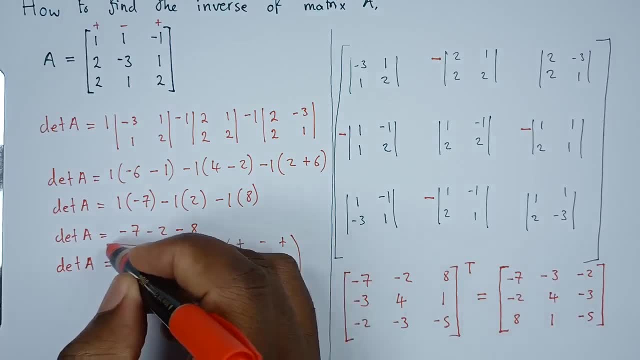 matrix. so remember, we have the determinant, now we have the adjoint, so the adjoint is found when you transpose. so let's just write it properly here. so the adjoint adjoint of A is equals to the matrix. we just from finding which is negative, 7, negative 2. 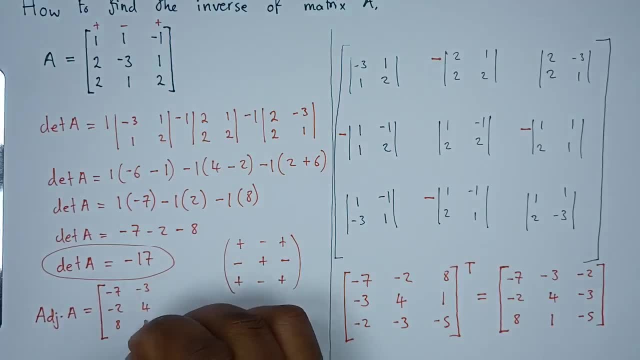 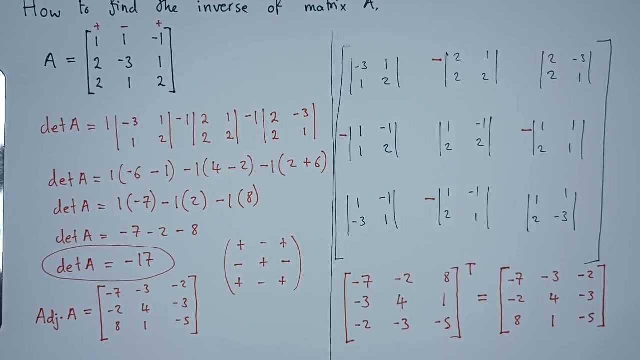 8 negative 3, 4, 1 negative 2 negative, 3 negative 5. so we have adjoint as well as the determinant. so this is how we find the expression for this. let's conclude: okay, so this is what you have. this is the determinant and the adjoint. so to: 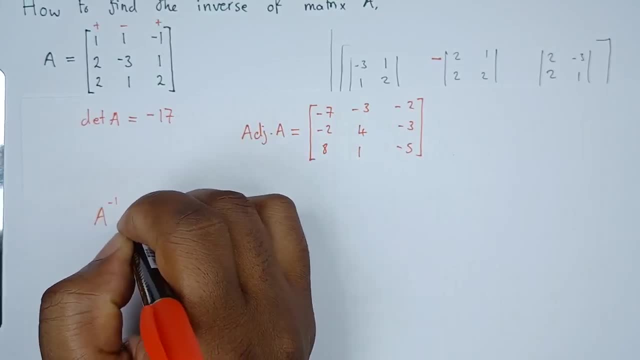 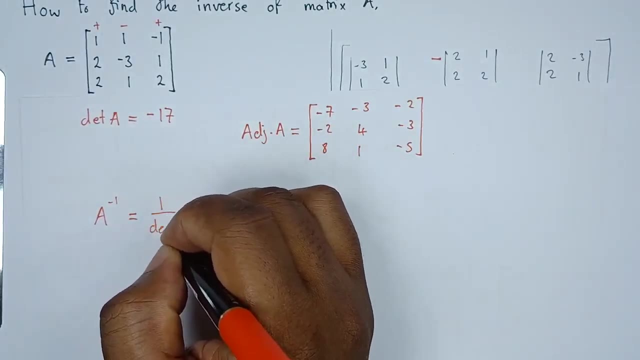 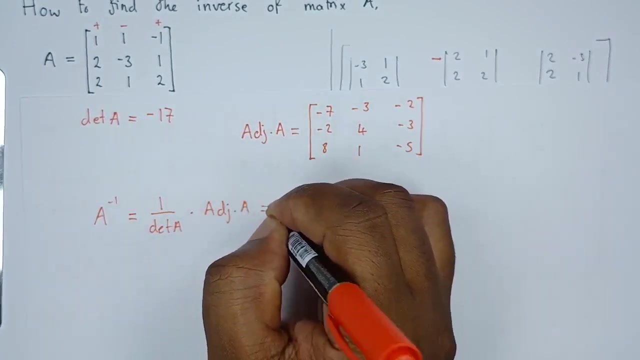 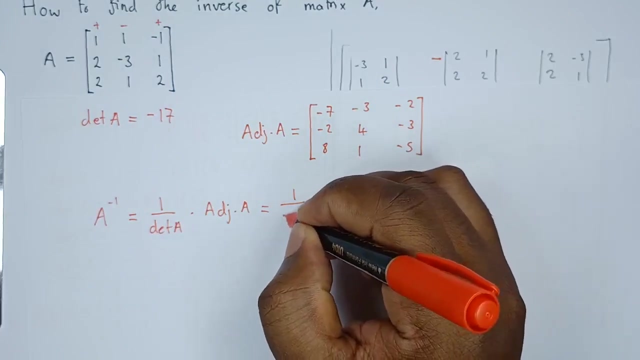 find the inverse. we can say inverse of A. so the inverse of A will be given as A, A. the formula is 1 over the determinant of A multiplied by adjoint of A. so the inverse will be equals to 1 over the determinant. remember it's negative 17. 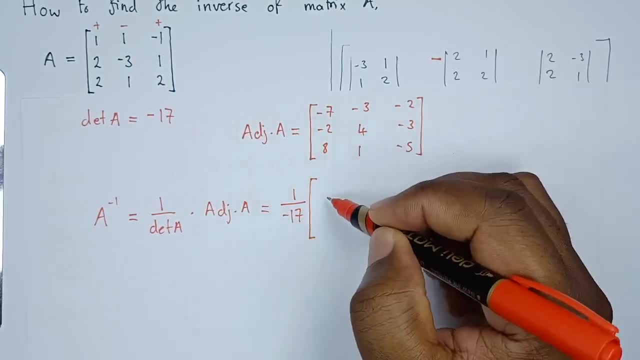 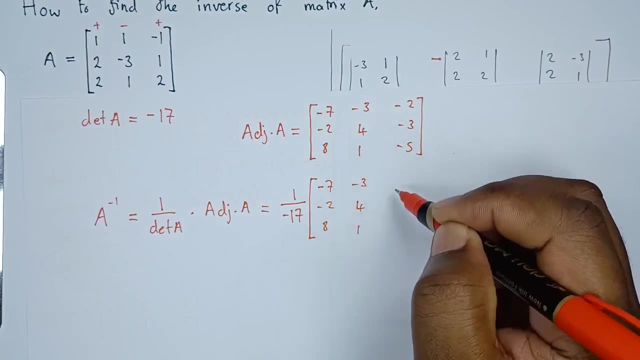 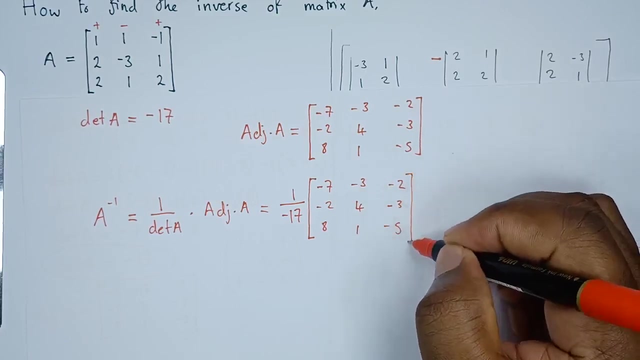 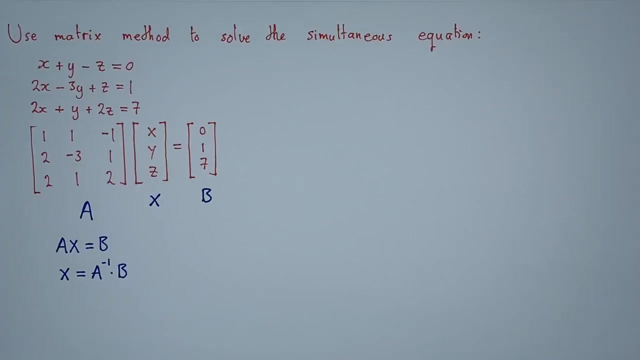 the adjoint, which is the matrix we found, is negative 7. negative 2, 8. negative 3, 4. 1 negative 2. negative 2, negative 3, negative 5. okay, this is our inverse. okay, so now that we have found the inverse of matrix A, let's write it here. we can say: 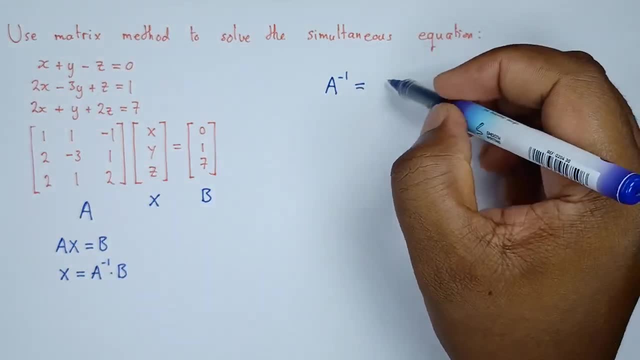 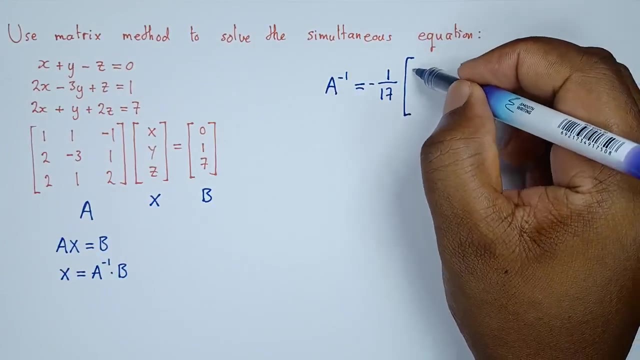 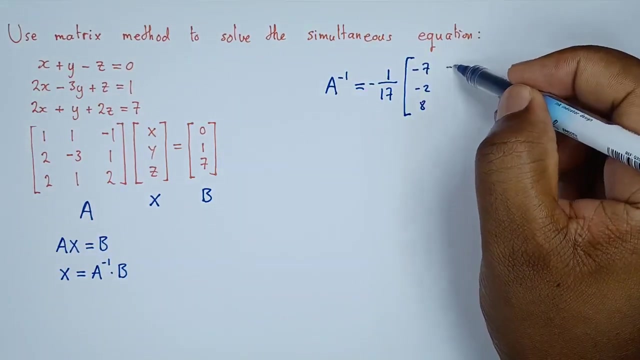 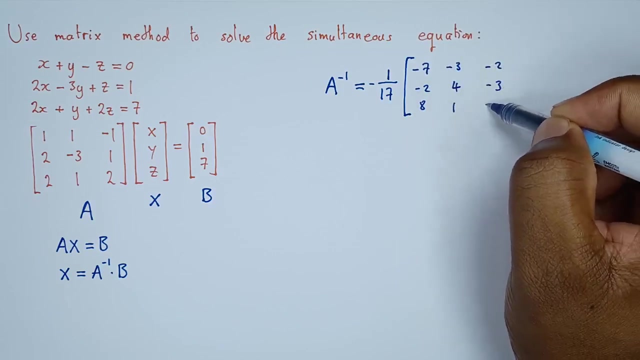 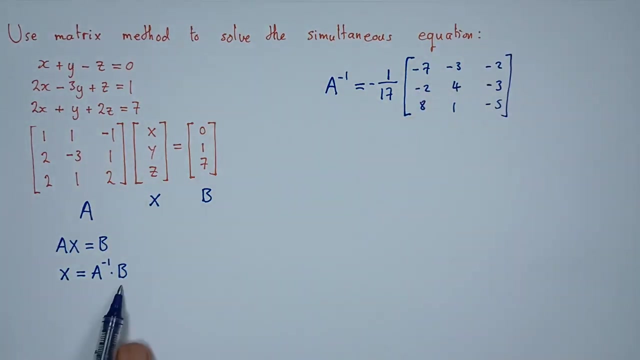 inverse of A is equals to, we said, 1 over 17- this is a negative here- multiplied by negative 7, negative 2, here we have 8. then minus 3, or 1, negative 2, negative 3, negative 5. okay, so that is our inverse matrix. so we shall multiply the inverse with B to 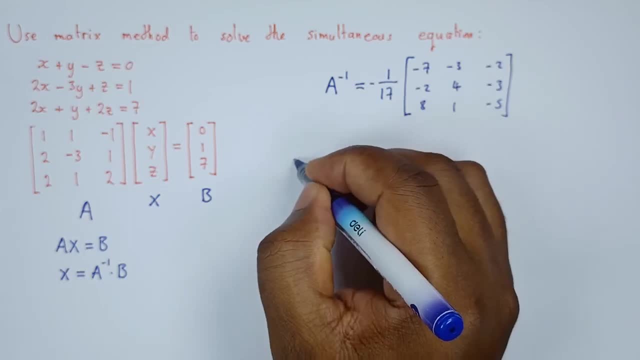 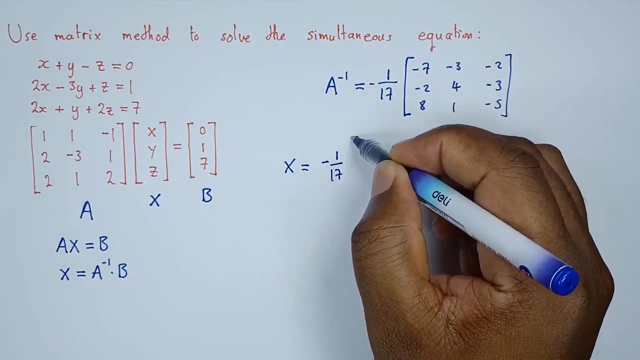 find the value of X. so I'm going to write it like this: X will be equals to the inverse 1 over 17. even if you multiply 17 with everything inside, you get fractions. so it's just better to leave this 1 over 17 outside the bracket. 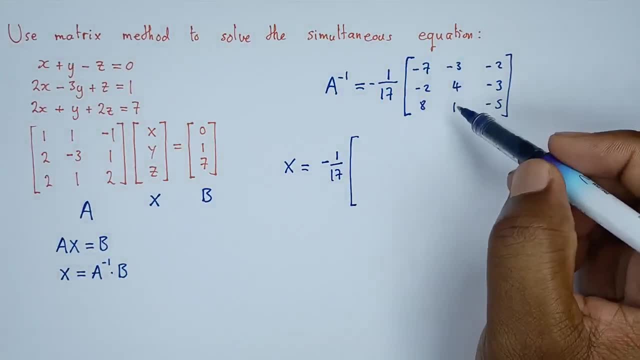 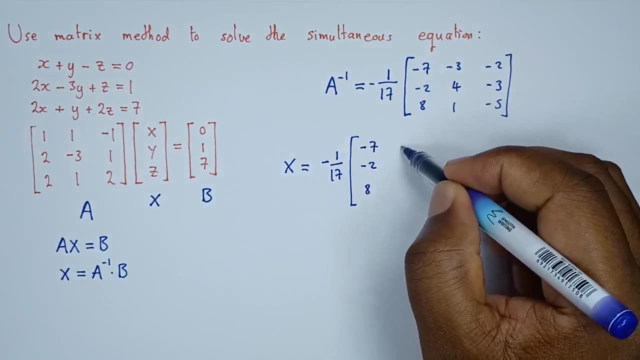 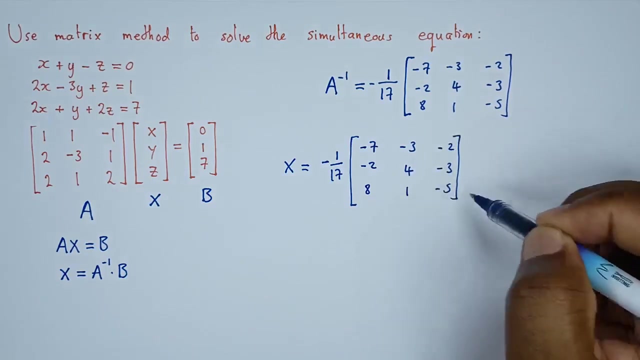 then we'll use it on the final step. so the inverse- remember I want inverse- of A. we have negative 7, negative 2, 8 negative, 3, 4 1 negative, 2 negative 3 negative 5 negative 3, 4 1 negative, 2 negative, 3 negative 5. 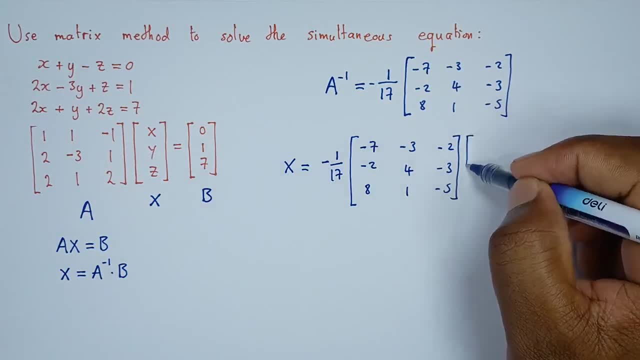 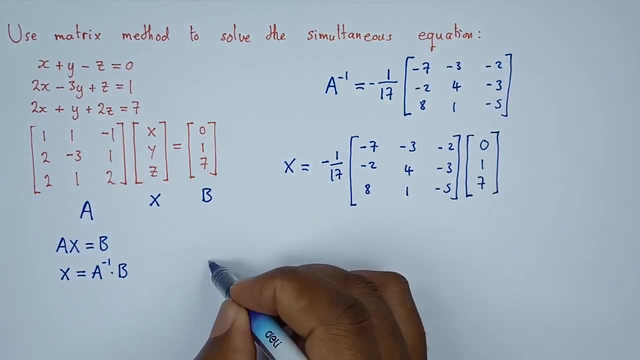 multiply with matrix B, which is this one here. matrix B is 0, 1, 7. okay, so let's multiply the two matrices. so I'm multiplying the two matrices. remember we still have negative 1 over 17 outside the bracket. now this matrix is a 3 by 3. 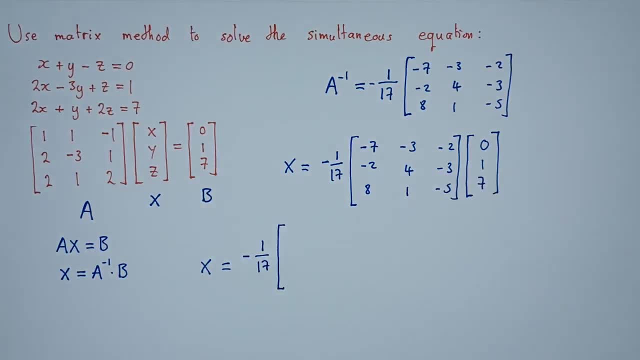 this matrix is a 3 by 1, so our final result should be a 3 by 1. so row by column: 7 negative 7 times 0, we get 0. negative 3 times 1. we get minus 3. negative times 7 get minus 14. 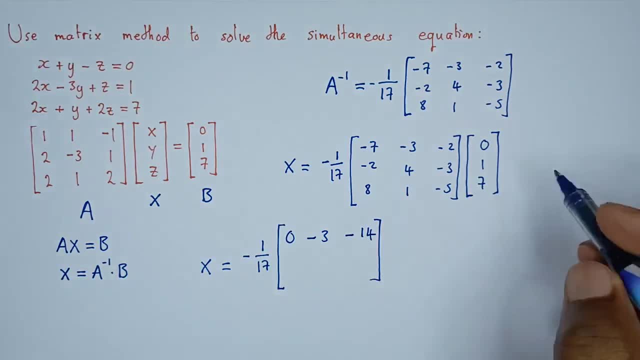 we go to the next row. negative 2 times 0, that's a 0. 4 times 1, that is a 4. negative 3 times 7, we get negative. point 1: 8 times 0, that is a 4 – 5. 2 x 4 is the third one x 3 minus 4 times 4, we get 4 x – 7. Todos los segundos, hipster. and negative three times 7-14, we get 0. we get minus four negative three times seven. we get negative point one negative 3 times 7 곧. We go to the next row: negative two times zero. that is a 0, 4 times 1. that is a 4 negative 3 times 7 곧.